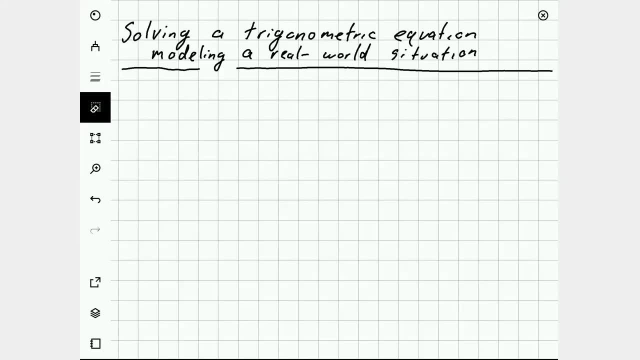 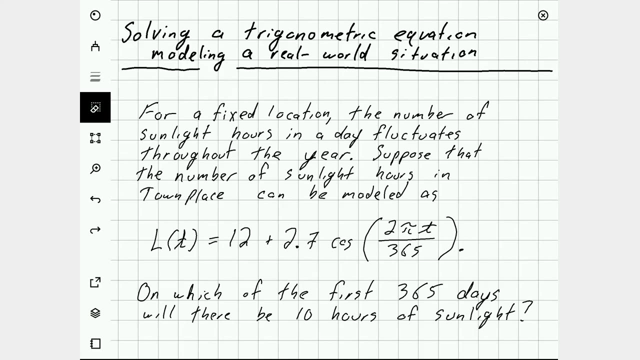 Solving a Trigonometric Equation: Modeling a Real-World Situation. We already know how to solve a trigonometric equation, so let's get the real-world situation here so we can model it. For a fixed location, the number of sunlight hours in a day fluctuates throughout the year. Suppose 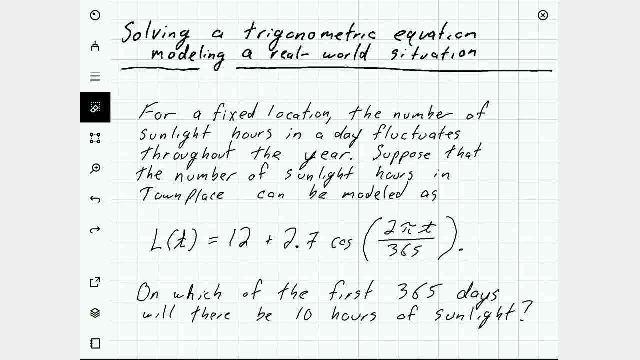 that the number of sunlight hours in town place can be modeled as this function. L of t equals 12 plus 2.7 times the cosine of 2 pi t over 365, where t is counting the number of days since June 10th of this year. 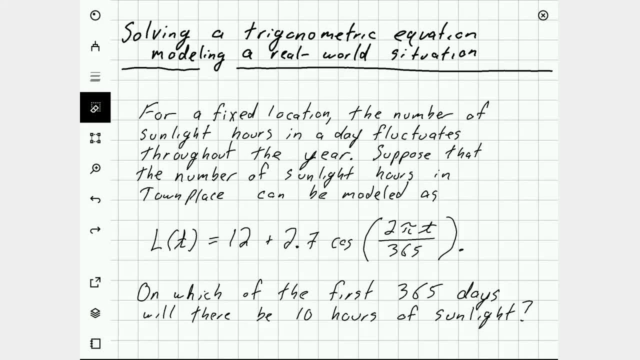 On which of the first 365 days will there be exactly 10 hours of sunlight? Well, probably there will never be exactly 10 hours in one particular day, but we'll get as close as we can in the first 365 days. So a lot of information here, most of it fairly useless to us. 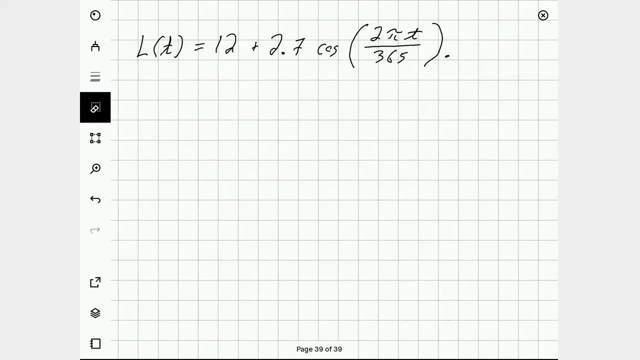 beauty of mathematical modeling. So let's take a look just at this function And remember we're looking for the day at which there are 10 hours of sunlight, So I want to set this equation equal to 10.. And we can do some pretty simple. 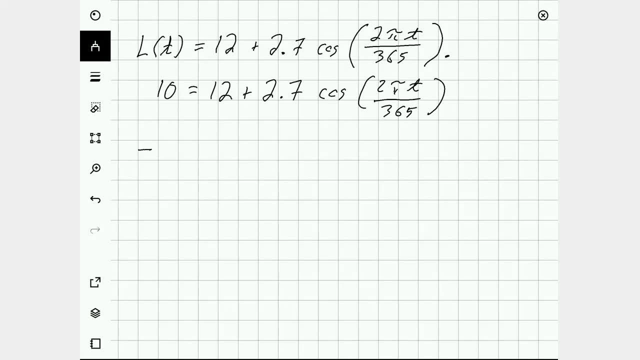 rearrangements here. subtract 12 on both sides of the equation. So I want to subtract 12 over 2.7.. Negative 2 over 2.7 is the cosine of two pi t over 365.. Now here before I continue onward. 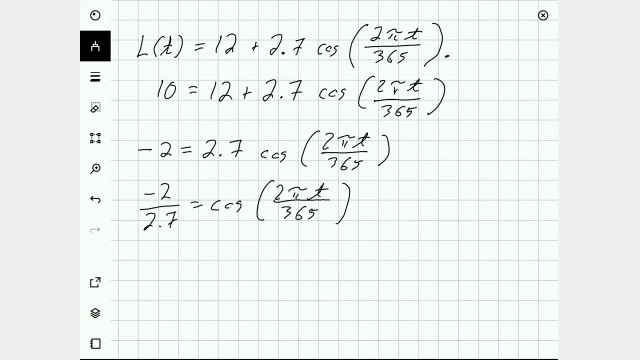 to think a little bit about my domain. I was asked to find the days in the first 365, which means that zero is less than or equal to T is less than 365. Or, to play it safe, we might want to do less than. 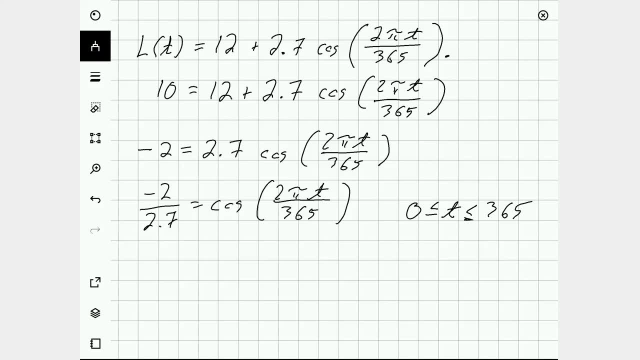 or equal on this side as well. Now my argument on my function here: two pi T over 365.. If I multiply all three sides of this inequality by two pi and I divide all three sides of this inequality by 365, I get that the argument of cosine. 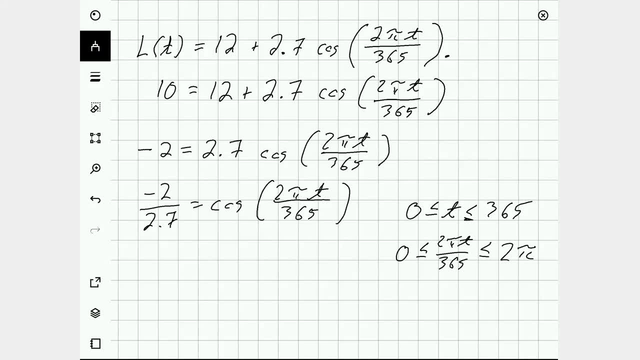 is somewhere between zero and two pi, Very convenient. These are the places that we normally are looking for when we're looking at solving trigonometric equations. So my next step is going to be to do a U substitution, And the point of a U substitution is just to find: 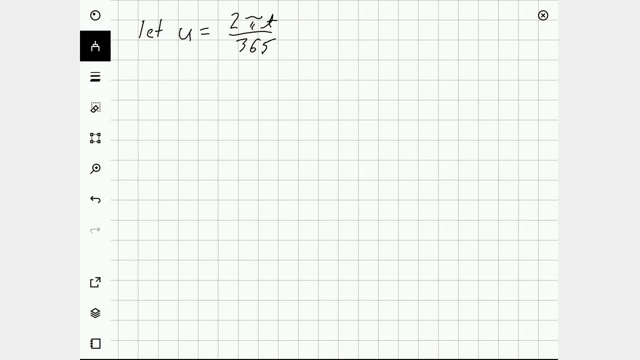 a new way of writing your argument of your function, so it's a little bit easier to work with. I like this particular substitution because solving trig equations, where I'm looking for solutions between zero and two pi, is kind of the standard of solving trig equations. 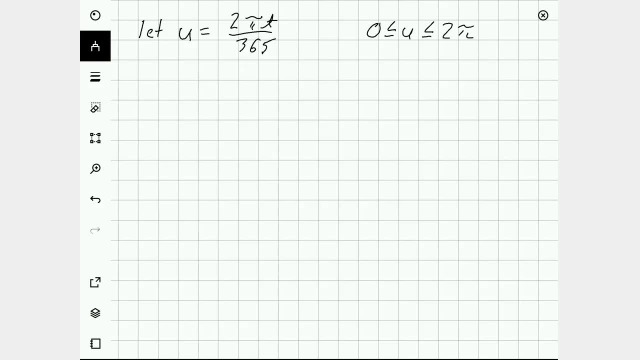 I also greatly prefer solving trig equations when I'm solving for the argument of the function and not other stuff going on. So negative 2 over 2.7 is the cosine of u. I will grab out my calculator at this point and evaluate the inverse cosine. 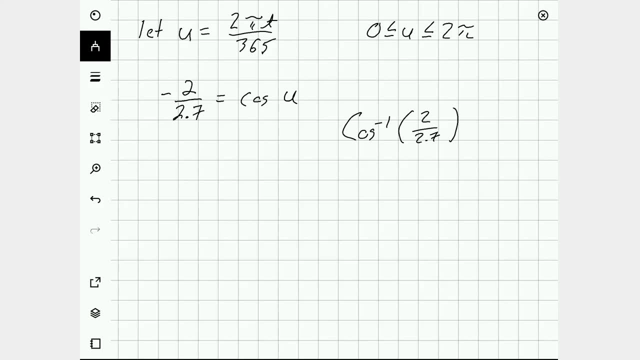 of 2 divided by 2.7.. As I often do when I'm working with my trigonometric functions, I'm going to evaluate the sine of 2 divided by 2.7.. So I'm going to activate the trigonometric functions and then I'm going to count the Fourier Lokians. 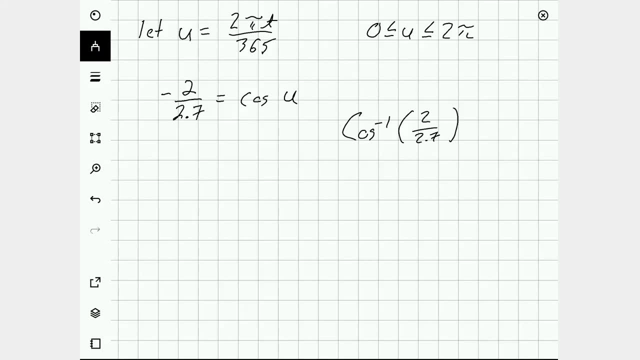 ignore the fact that I have a negative value here and deal with that. after I find the value of the reference angle, I get here that my reference angle is going to be 0.7, well, around to the nearest thousandth, 0.737, and that's in radians. 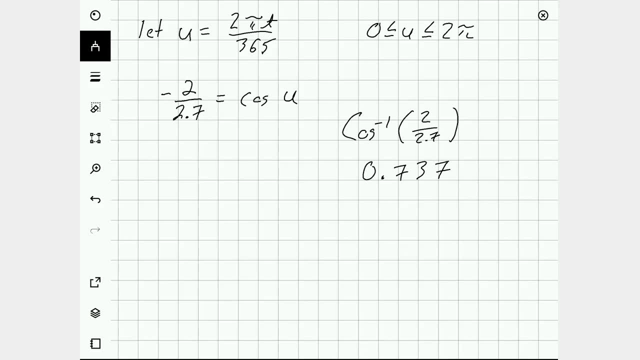 I also know, looking at this, that I'm dealing with a negative value of cosine, and negative values of cosine occur in the second quadrant and in the third quadrant, So I might have that as 0.737, and I might have that as 0.737,. 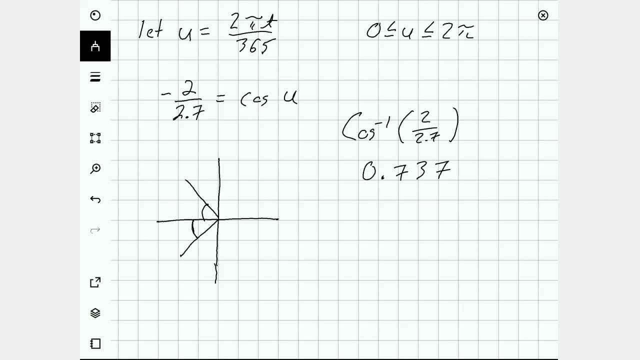 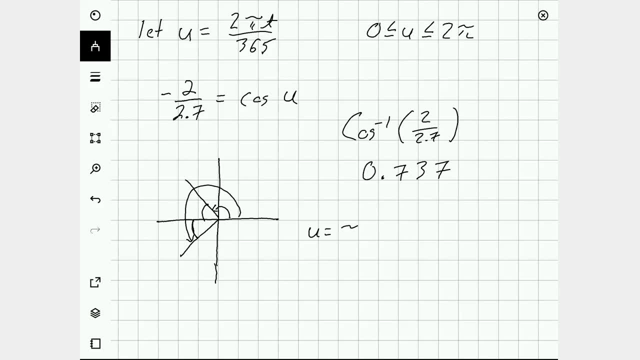 Either it's going to be pi minus 0.737, or it's going to be pi plus 0.737.. Those come out at 2.405, or 3.805.. Or 3.805.. These are the two possible values for u between 0 and 2 pi. 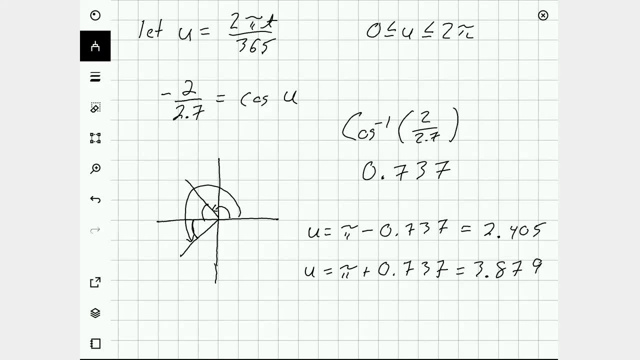 And, as we saw on the previous page, if we keep u between 0 and 2 pi, that will ensure that t is between 0 and 365.. So now let's grab all this information. I know that u is 2 pi t over 365, and I've figured out that u is either 2.405, or u is 3.879..